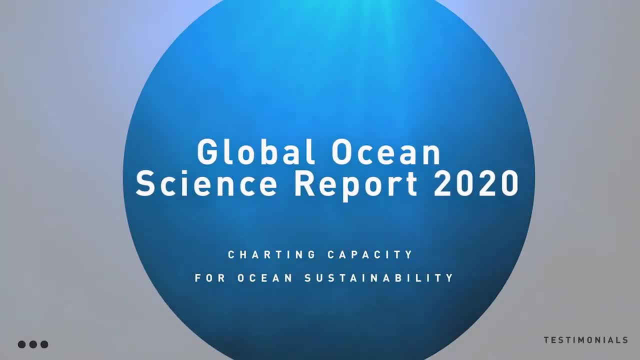 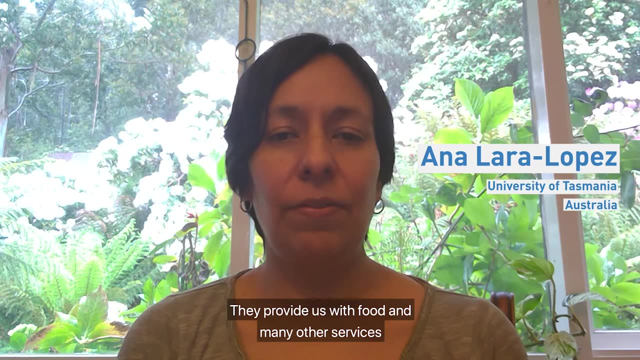 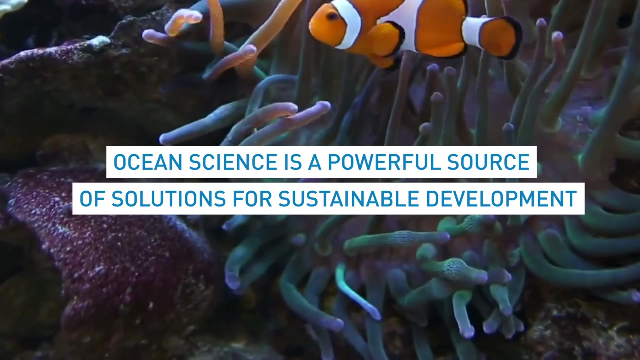 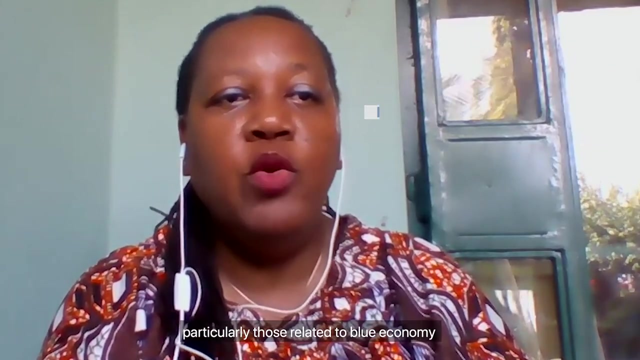 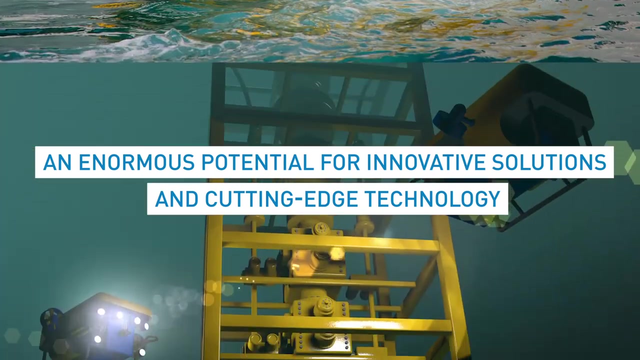 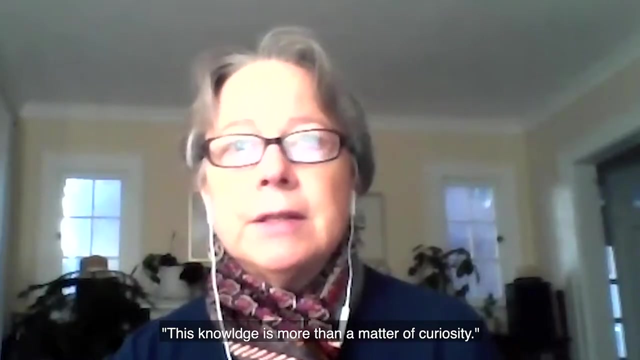 The oceans are essential for life. They help us regulate our climate, they provide us with food and many of the other services that are essential for our well-being. Ocean science is making a contribution to in-country dialogues, particularly those related to the blue economy and the achievement of SDG 14 targets. 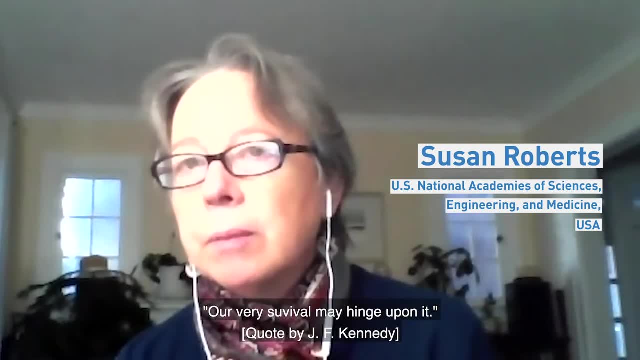 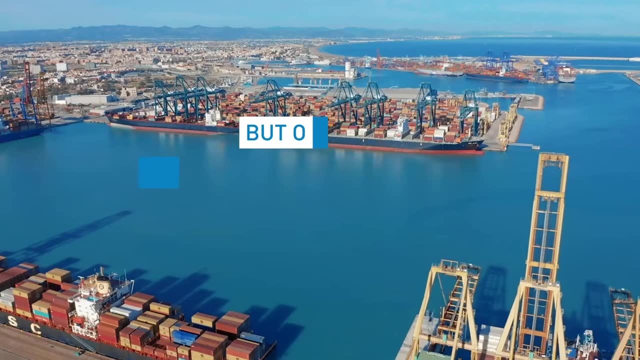 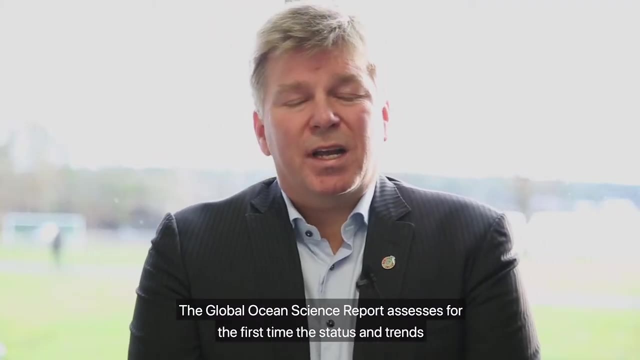 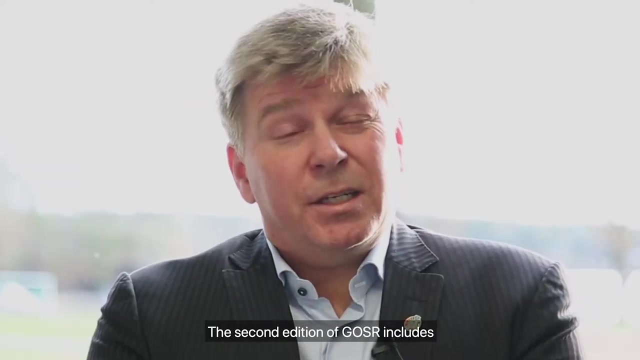 This knowledge is more than a matter of curiosity. Our very survival may hinge upon it. Global Ocean Science Report assesses for the first time the status and trends in research capacity around the world. The second edition of Global Ocean Science Report includes new measures, updated information. 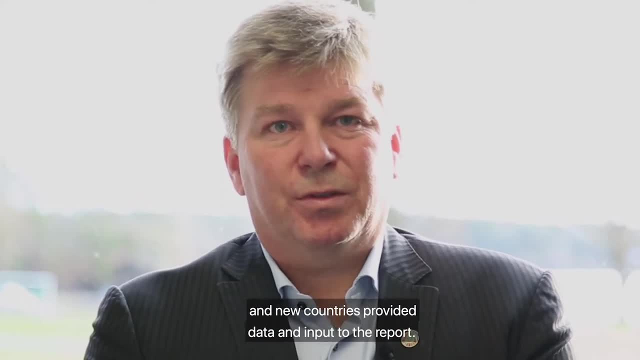 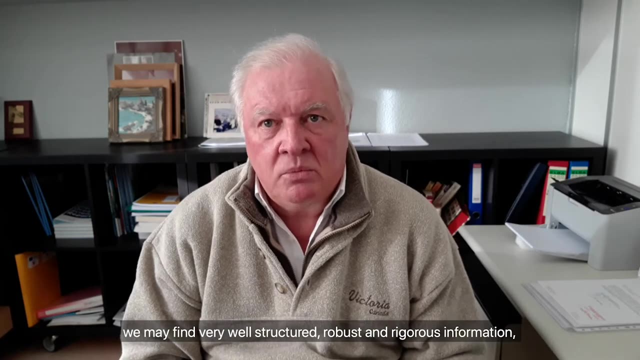 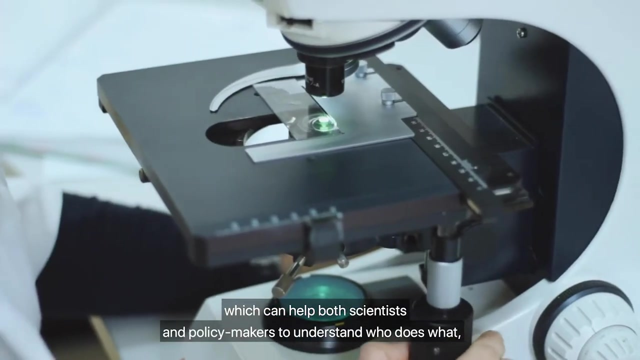 and new countries provided data and input to the report. In the Global Ocean Science Report you can find very structured, very well-made, very rigorous information that can help not only scientists but also the people involved in policy and decision-making to understand who does what, what products are obtained. 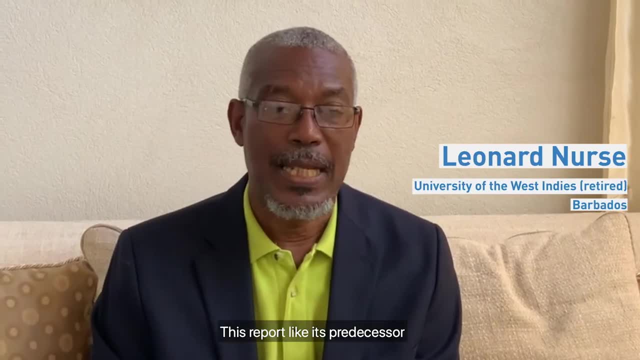 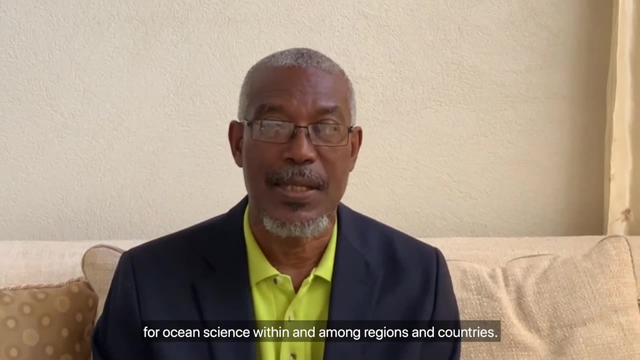 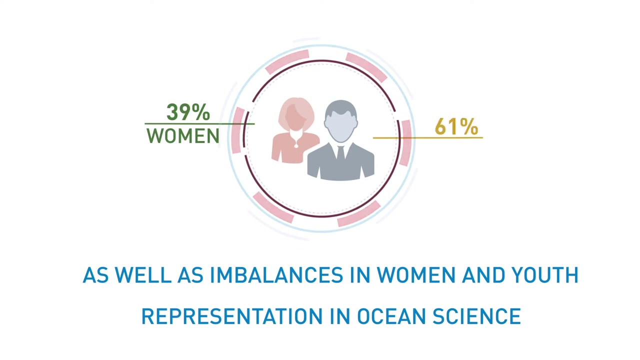 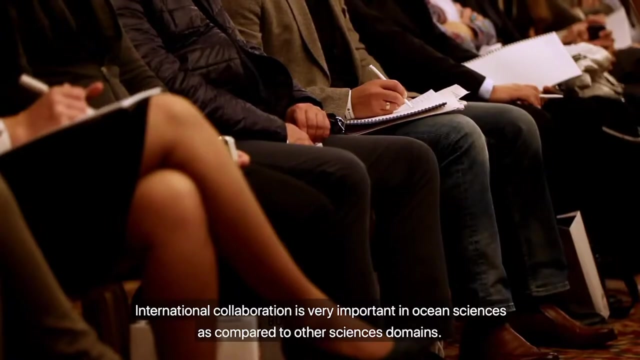 what resources are consumed, etc. etc. This report, like its predecessor, continues to underscore the uneven distribution and allocation of funding for ocean science within and among regions and countries. International collaboration is very important in ocean sciences. Also, as compared to other science domains, the more international collaboration we see. 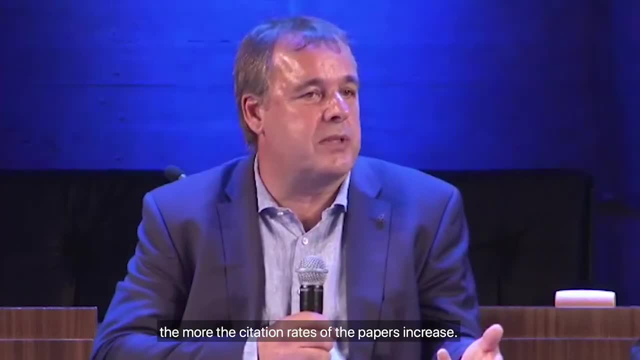 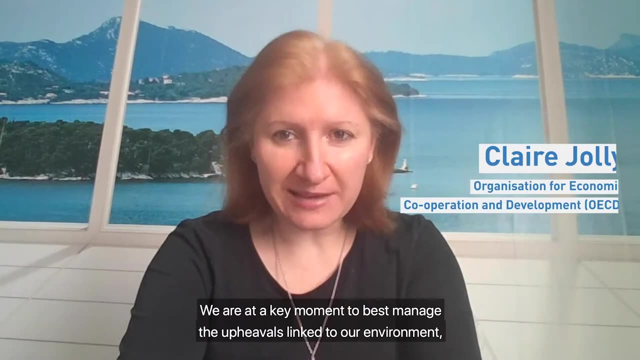 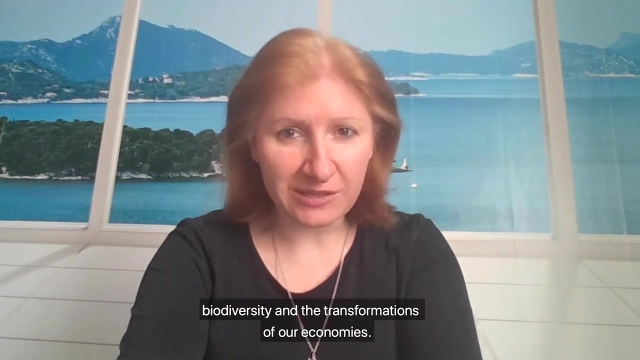 in publications, the more the citation rates of the papers increase. We are at a key moment to manage, at best, the disruptions to our environment, to biodiversity and to the transformation of our economies. Science and the oceans have a key role to play.